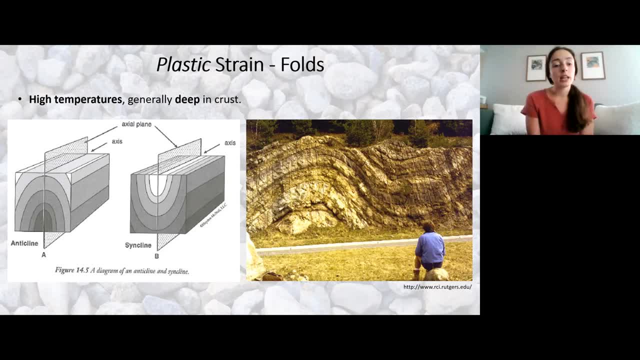 be able to fold without breaking, And so when you get folds, you'll get either anticlines or synclines. There are other types. For the purposes of this video, it's just no anticline and syncline. Anticline is like an upside down u-shape and syncline is a upside up u-shape, And it's 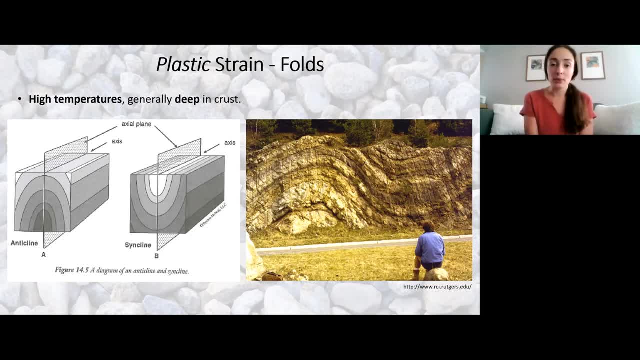 important to understand which one you're looking at when you look at an outcrop, because that will help you understand the age of the rock layers and then you can better interpret what happened there and the geologic processes that went into causing that feature. Now brittle deformation is. 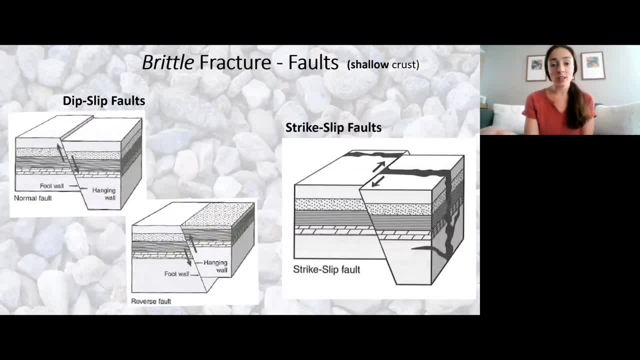 a little different. Instead of folding, you'll get breaking, or what we call faults, And so brittle deformation, we know, happens shallower in the crust, and this is at cooler temperatures, and the rocks are harder and less deformed. And so when you get folds, you'll get more deformed. And so when you 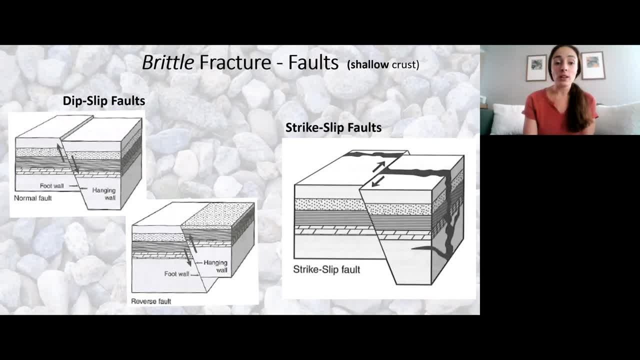 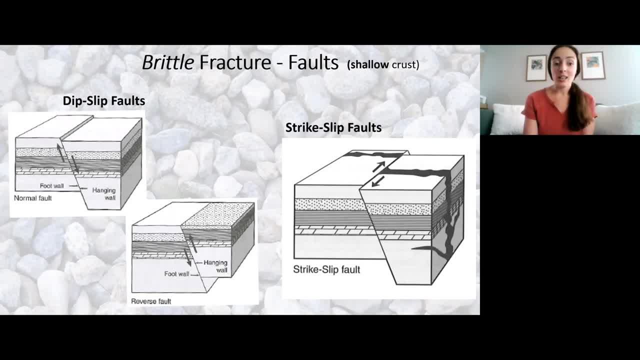 faults we'll be talking about are dip slip faults, specifically normal and reverse faults, and strike slip faults. Now, the types of stress that you're getting in each of these situations is important to understand. So when you have normal fault, you're going to have a tensile stress and 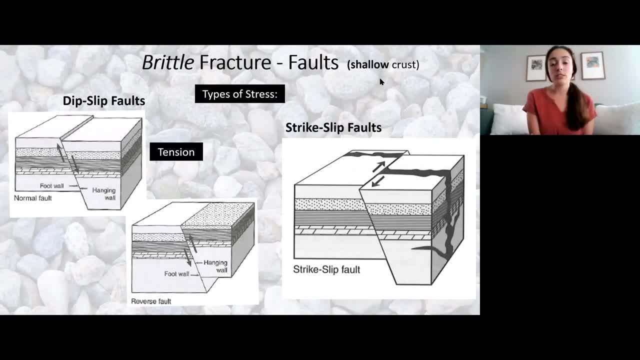 this is when things are pulling apart. You'll see this again when we talk about divergent plate boundaries, When you have a reverse fault that's formed from compressional stress or over-stress or over-stress, You'll see that this is a very common situation where we're 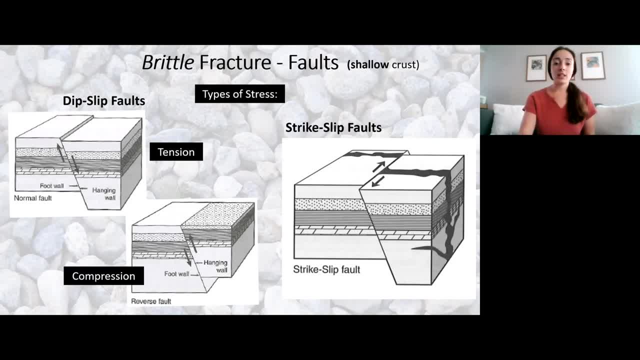 pushing together, And you'll see this in convergent plate boundaries. Now there's another type of compressional fault that's important. that is technically a reverse fault, but we call it a thrust fault. It's just basically a really shallow reverse fault. And then, lastly, you have strike. 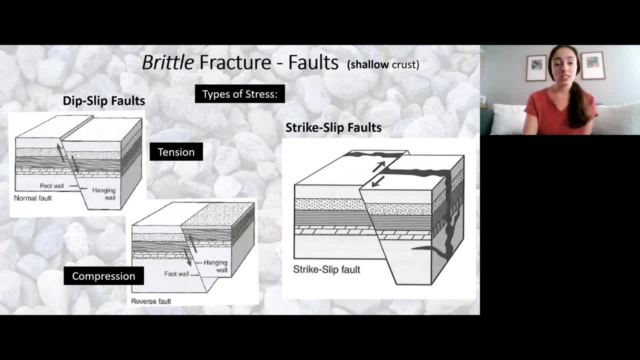 slip faults which form from neither compression nor tension, but shear, Shear stress is going past one another rather than pushing or pulling apart from one another, And this causes strike, slip faults And you will see this shear strain again when we talk about transform plate boundaries. So 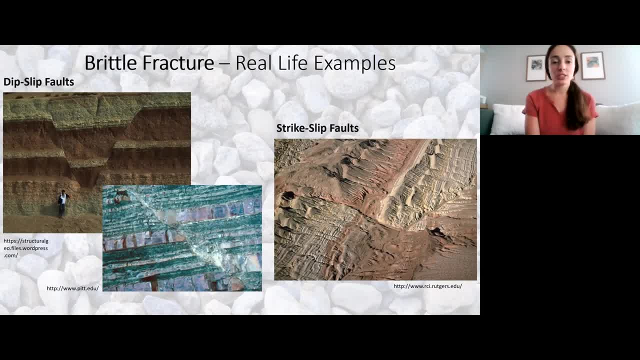 just to give you some real life examples of these rock features. you have this beautiful dip slip fault showing in the first picture. Basically, the tension or extension of those layers pulling apart caused this block to drop down And you can see that in the faults, how they line up. it dropped. 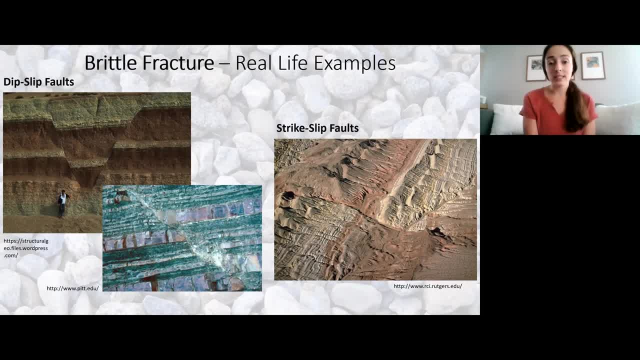 down. And then you have a reverse fault, shown in the second dip slip image. This is identifiable by the strata in the middle Showing how it pushed up. And lastly, we have the strike slip fault, which is seen in the far right. 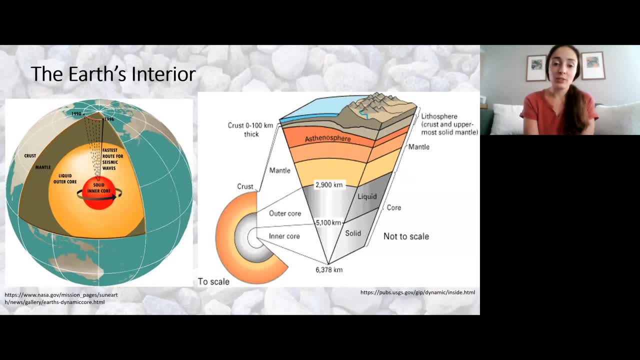 picture. So next I want to move on to Earth's interior. We're not going to go into detail on each depth of each layer and breaking down the mantle into all the different things that it is composed of, but we're just going to do the basics. Basically, we have a solid inner core, a liquid. 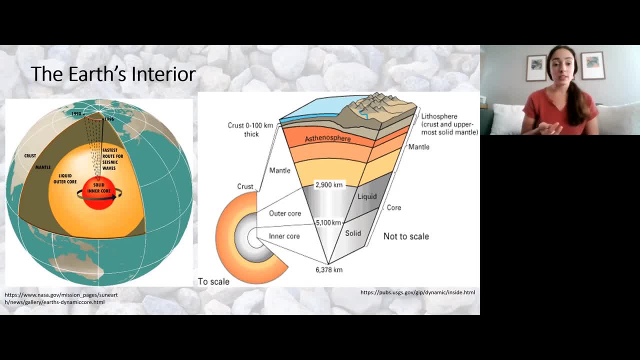 outer core, a mantle, and then our crust. Now you might be confused, because the lithosphere and the mantle overlap. Well, that's because the lithosphere and the mantle overlap. So the lithosphere and the mantle overlap is part of the fuselage, Because the ludosphere not only includes the crust but also. 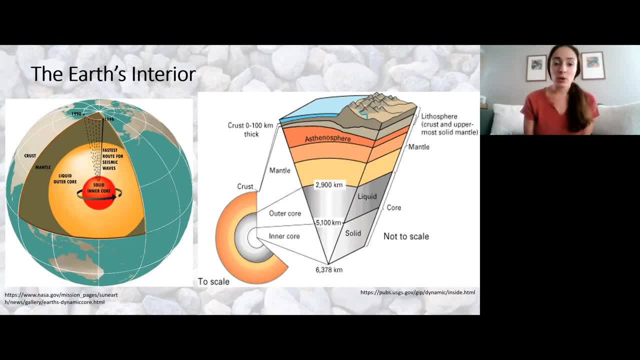 the uppermost part of the mantle And this is really important when we're going to get into plate tectonics. So this you need to understand: Lithosphere is crust and mantle, asthenosphere, is just mantle but not the uppermost part, The uppermost part of the mantle below the upper uppermost part. 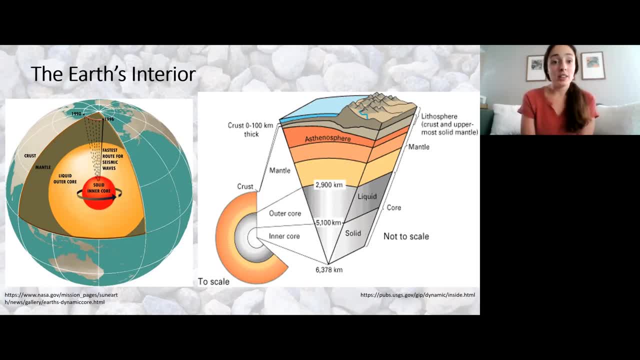 of the mantle. Okay, I made it worse. We'll move on Not to confuse you more. but there's also something called the moho discontinuity. There's a little bit of discontenitation with this moho discontinuity, for 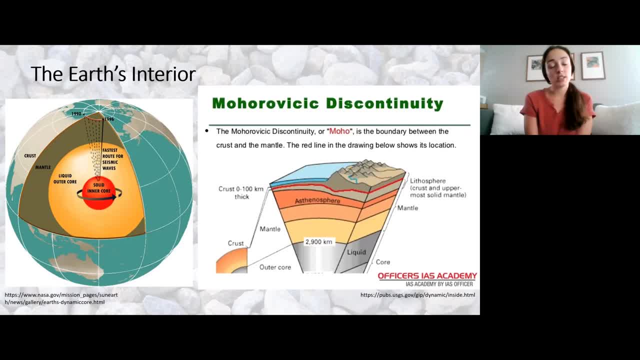 the lateral support which is completely pondering This moho discontinuity marks the pope in any super, the boundary between the crust and the mantle, And this is why we can't just say that the lithosphere is the crust and then the mantle starts, because this boundary is really important. This marks the boundary where seismic waves change velocity and therefore the density of rock down at this level is changing dramatically, marking the beginning of the mantle And the lithosphere is what makes up the plates that plate tectonics is based on. I hope I explained that incredibly. 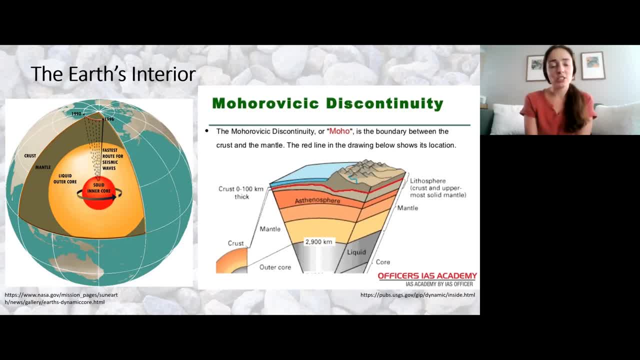 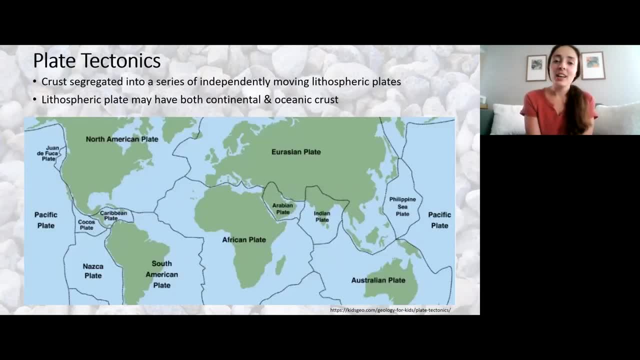 poorly. I'm sorry, But you can always rewind and interpret it for yourself. I'm just going to move on. Today is just not my day. So plate tectonics. hopefully I can explain this a little bit better. The lithosphere is segregated into what we call lithospheric plates, which finally something's. 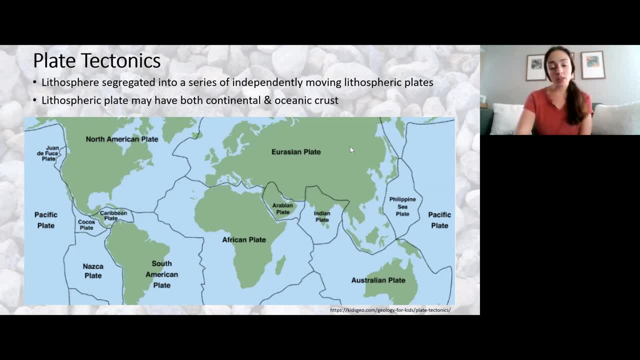 making sense right, And these plates can be made up of both continental and oceanic crust. As you can see in the picture, these plates don't necessarily follow the boundaries of continents, and that is because they are in the entire lithosphere, not just the crust part. So they 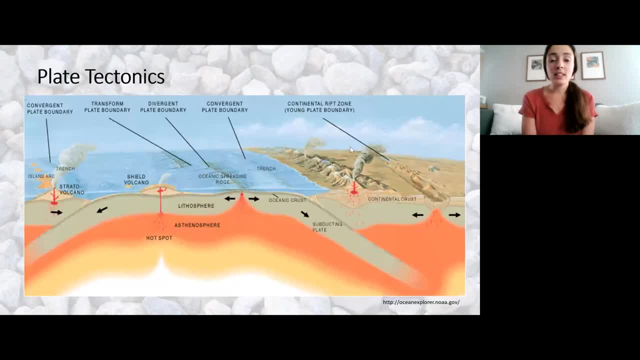 can host both oceanic and continental crust in the same plate And getting into how these plates move around, you might have noticed on the previous picture that a lot of the boundaries are close to where we have mountain ranges and volcanic activity, And this makes sense. 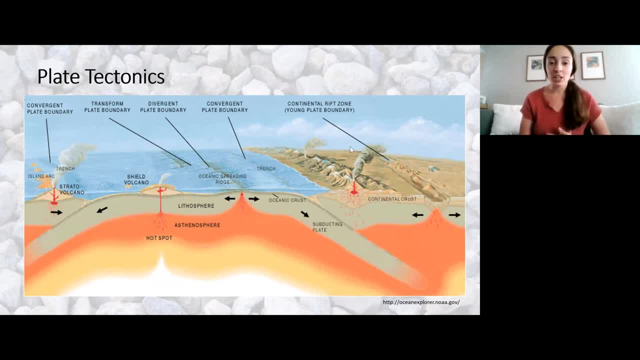 because in subduction zones or where an oceanic plate is going under a continental plate, this will cause volcanic activity to occur on the continental edge And that plate boundary is called an oceanic continental convergent boundary. You can also have divergent boundaries and 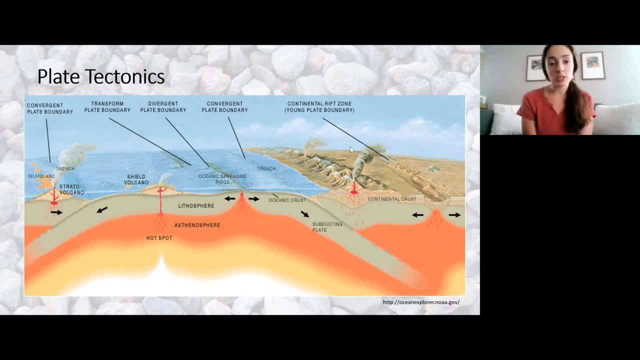 transform boundaries, Like we talked about in the brittle deformation slide: convergent is compressional stress, divergent is tensile stress. pulling apart and transform is shear stress rubbing against each other, And you can see here that both the subduction zones as well as the spreading 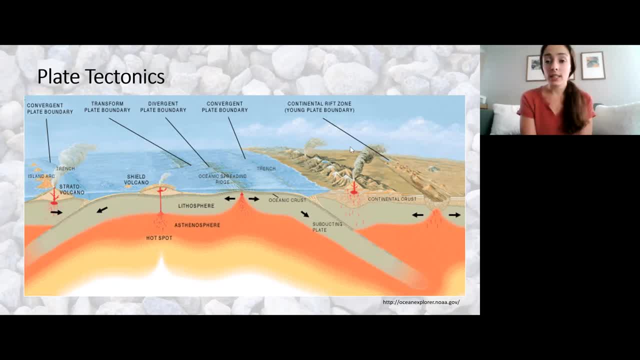 centers or divergent plate boundaries in the ocean cause volcanic and magmatic activity. You can also have what's called a hot spot, which is exactly what it sounds like: It's just a spot in a plate that has magmatic activity. because it's a hot spot, guys? 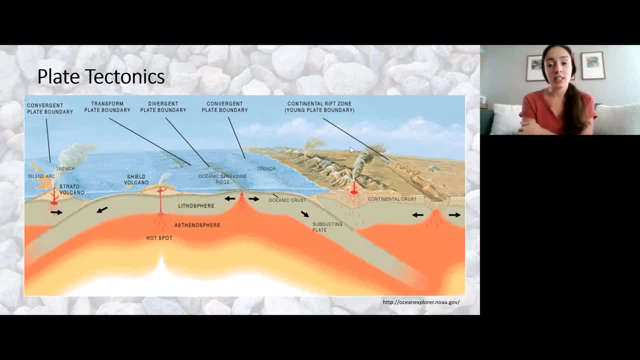 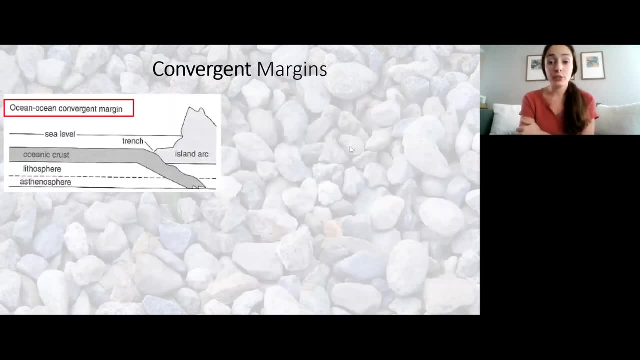 And that is typically what we see- starts divergent boundaries and we'll see that on the divergent slide. So let's get into the different types of convergent margins. You can have ocean-ocean convergent margins, in which subduction will occur to one of the oceanic plates and this will form 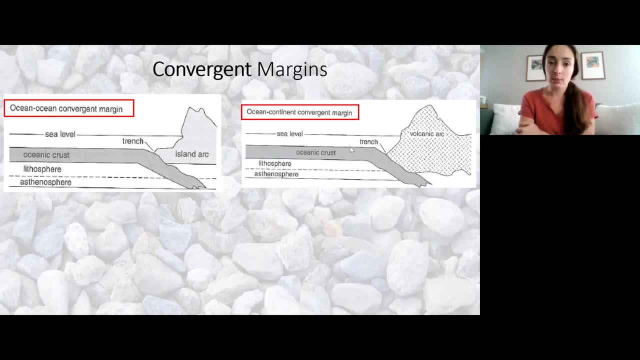 an island arc, Then you can have ocean continental, in which I talked about forms, volcanic activity on the margins of continents, And this also causes subduction of the oceanic plate, but it's always the oceanic plate. It's never a continent, because the continent's too buoyant and 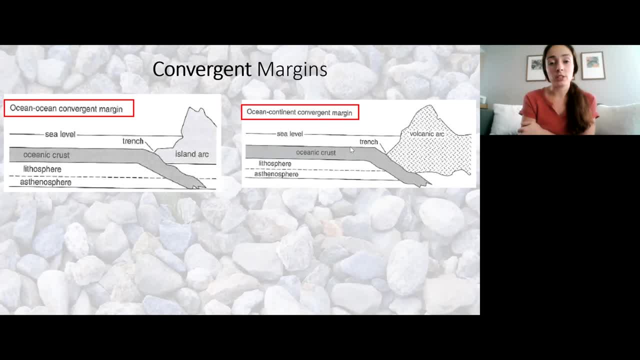 less likely to form an island arc. So you can have ocean-oceanic plates and this will form an island arc. It's less dense than the oceanic plate. It will never subduct under oceanic plate. Then, lastly, you have continent-continent convergent margins in which there is no subduction again. 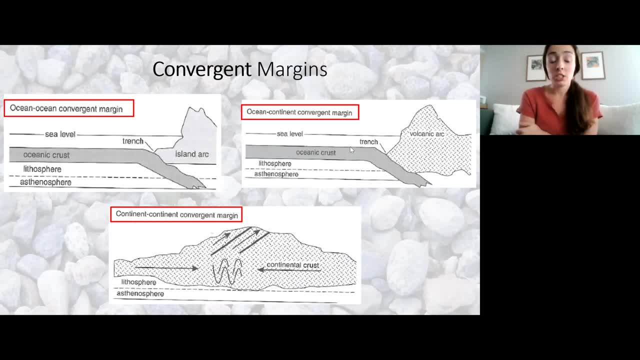 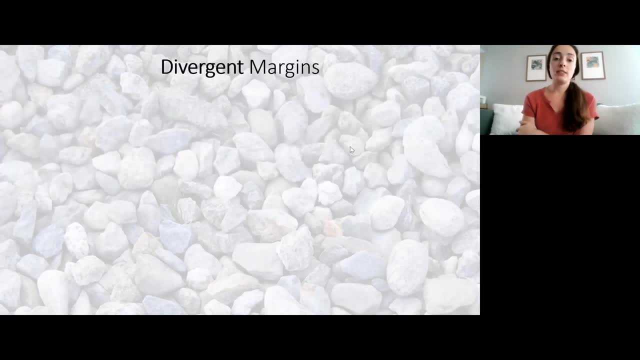 because these are not dense enough and so they just push into each other and crumble and crumble and make really really high mountains with really really thick crust, like the Himalayas, for example. Moving on to divergent plate margins, you will have ocean-ocean divergent margins, in which you saw 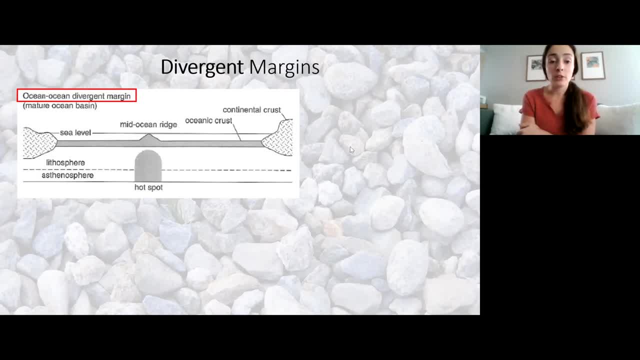 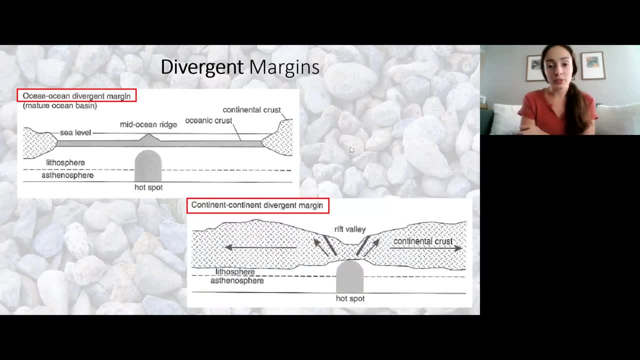 like the mid-ocean ridge, which is a spreading center because of divergence, and this divergence is typically started by a hot spot, and then you have ocean-ocean divergent margins in which you saw by a hot spot, as shown here. Then you can also have continent-continent divergence, which forms 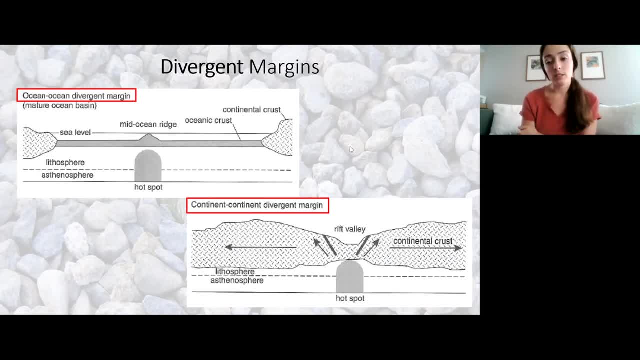 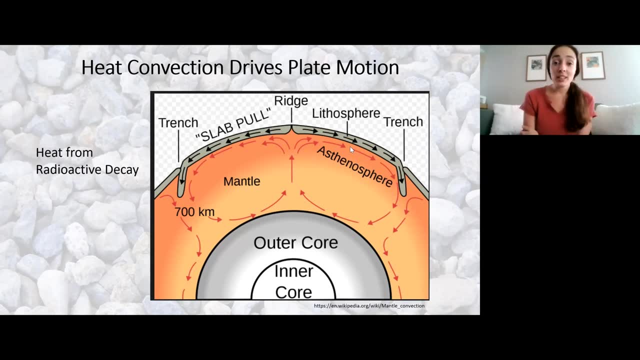 rift valleys. and again, these are often started by hot spots. Now, what causes plate tectonics? Well, plate motion is caused by heat convection. but what the heck is heat convection? Well, heat convection is caused by the movement of hotter, less dense material in the mantle. 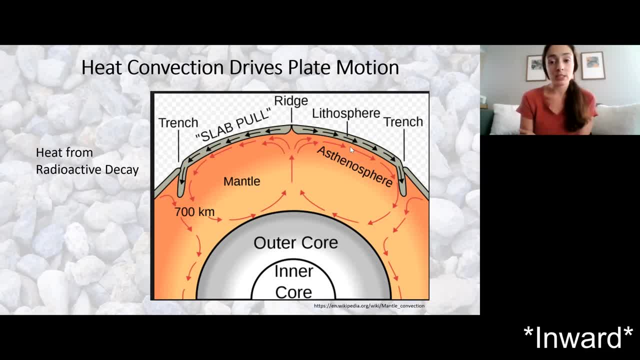 upward and the movement of cooler and more dense material downward in the mantle. And what causes the hotter stuff down low in the mantle to keep getting hotter? Well, it's radioactive decay. Ever since Earth was formed, radioactive elements have been decaying at a steady rate. 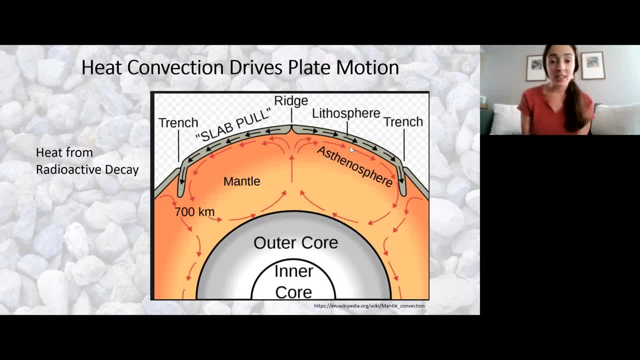 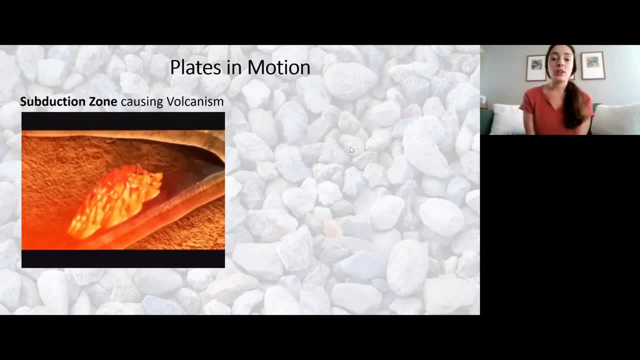 and many of those are still decaying today, And this has provided energy in the form of heat for Earth for billions of years. And lastly, I just want to show you a few animations that I found that I thought were really helpful for learning about plate tectonics. 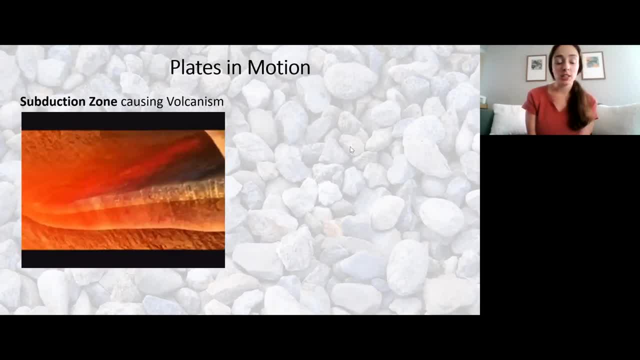 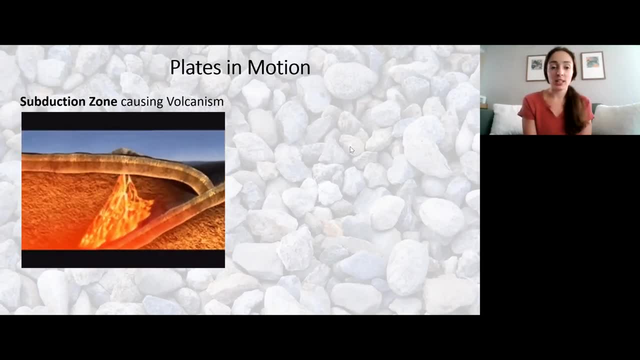 Basically, this is a subduction zone where you can see that the subducting oceanic plate is causing partial melting of the underlying mantle, which causes magma to rise and form volcanoes, And this is how we get volcanic islands and arcs. And this melting in the first place is largely due to the water content that is brought down. 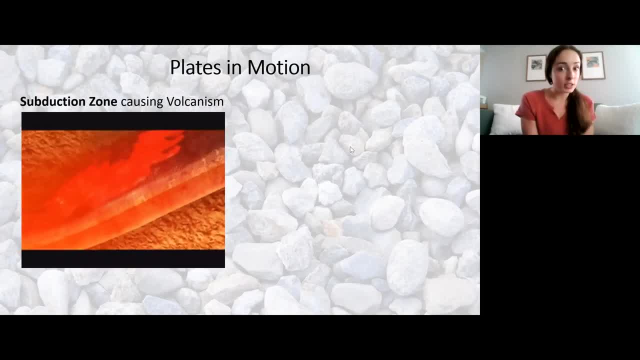 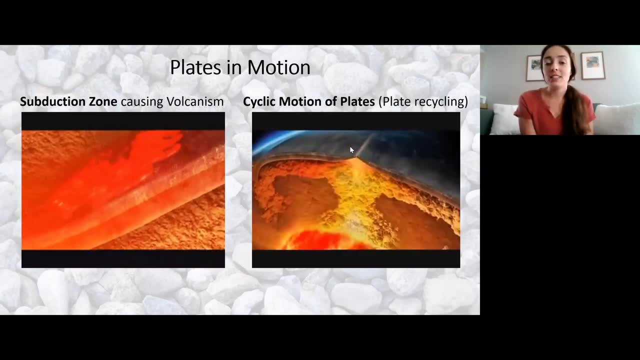 within the subducting plate, And this water content does wonders for melting the rock down there, And that's a big thing to remember. Next, this is one of my favorite animations for plate tectonics. Probably a little misleading just because it's happening so fast. 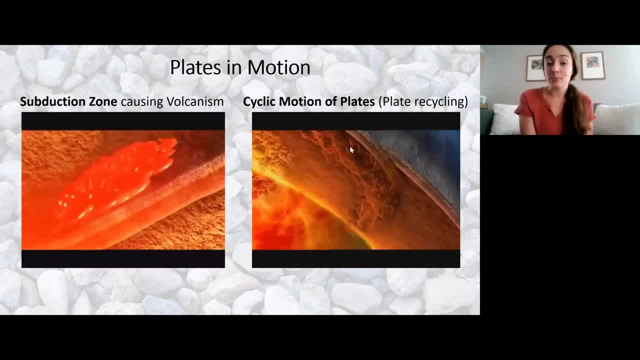 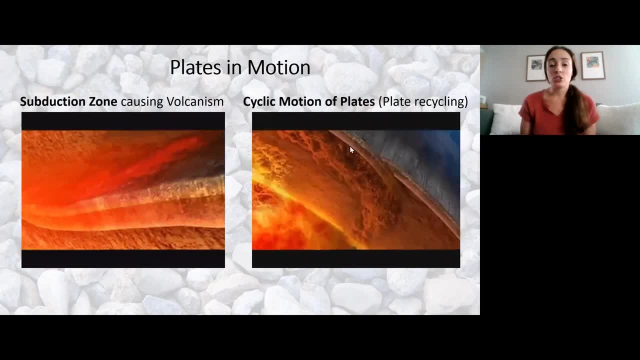 This does not happen this fast. But the reason I like this is because it shows it's cyclic, because new crust comes out of mid-ocean ridges Or spreading centers and is destroyed or brought back down into the mantle and recycled at subduction zones. 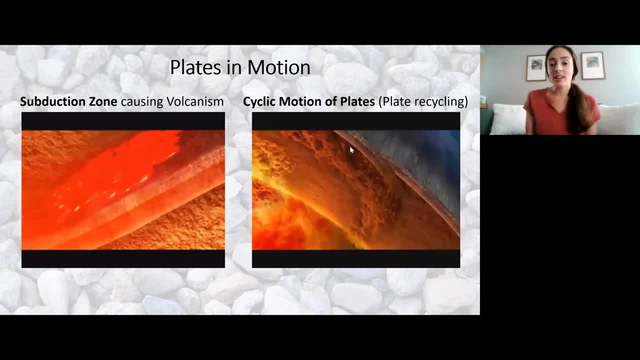 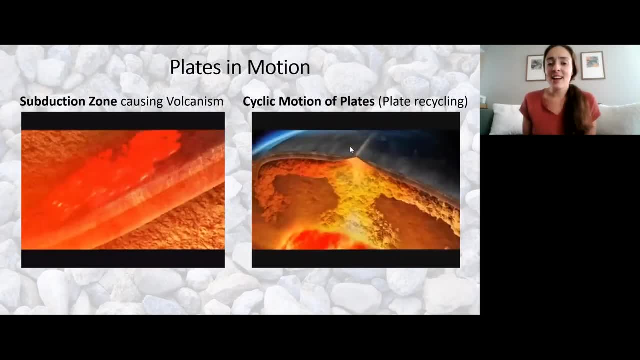 Although this is a really good animation because it shows the cycle really well And it shows both divergent and convergent boundaries, as well as mantle convection, I do warn you that the mantle is not like a cloud or whatever this image is showing. 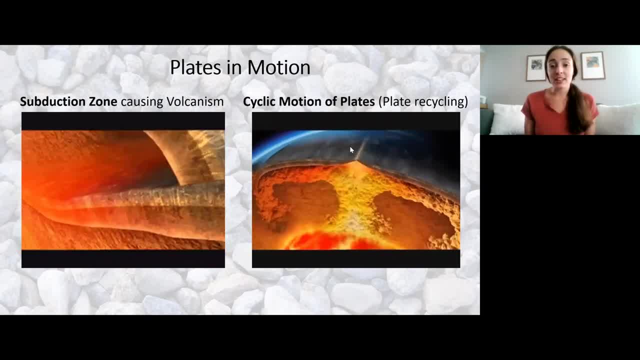 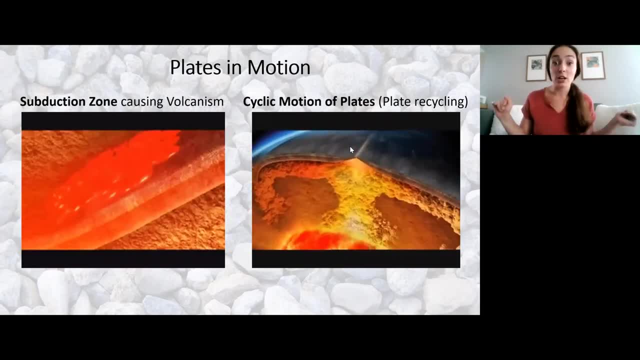 It is rock, guys. I mean it's not molten either, It is like hard rock. There is plasticity and things can move, Obviously, but it's not this fast. We're not all floating around on magma, basically. Okay with that. thank you so much for watching and I'll see you next time.